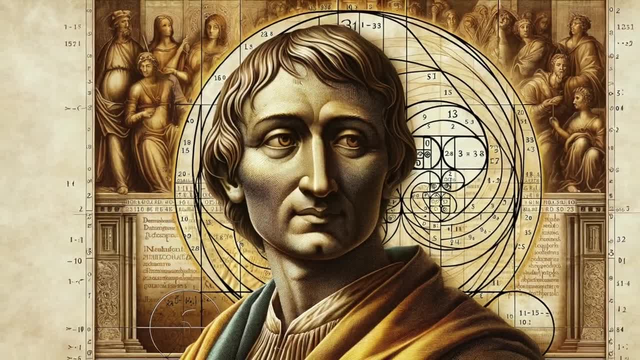 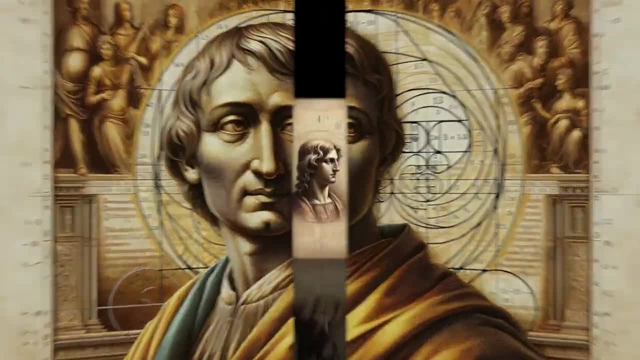 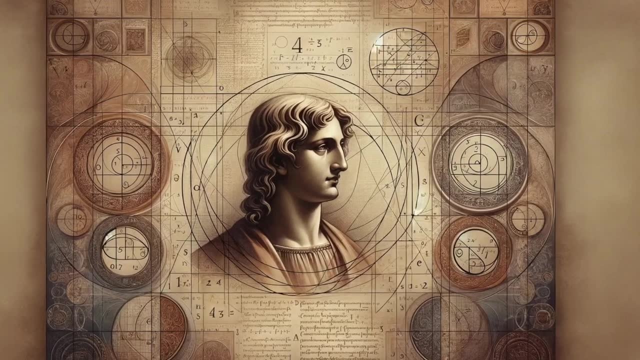 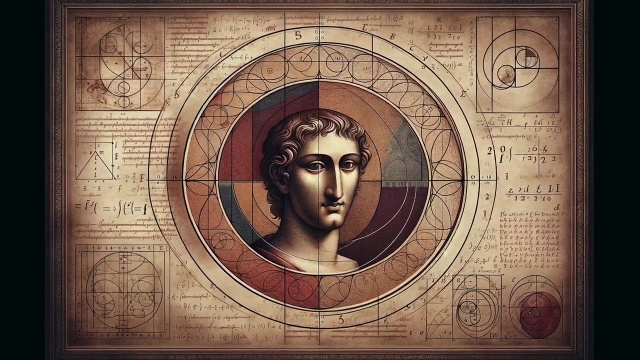 Hello and welcome. Today we will focus on the origins of Fibonacci and its fundamental theoretical principles, which play an important role in financial analysis. The origins of this mathematical concept actually date back to the 13th century and start with the Italian mathematician, Leonardo Fibonacci. Leonardo Fibonacci is known as a mathematician who lived 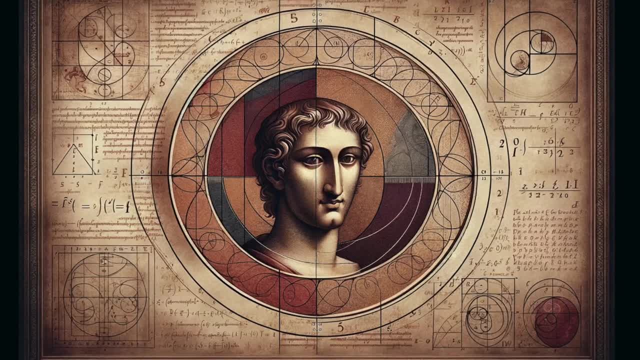 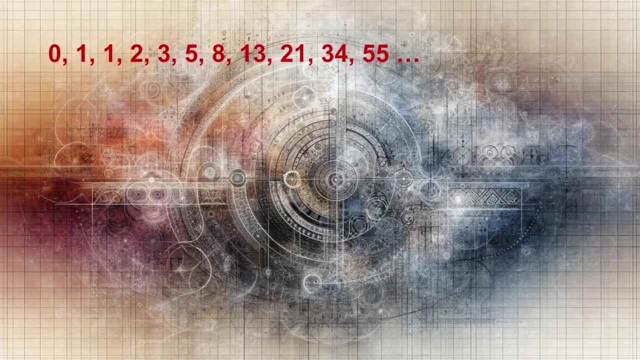 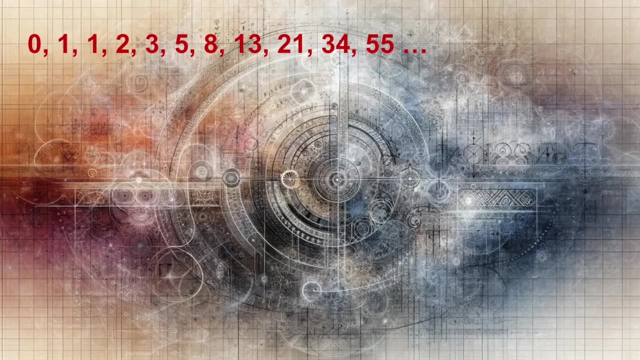 between 1170-1250.. One of his most famous works is the Fibonacci numbers, a number sequence that bears his name today. This sequence begins with 0 and 1, and each subsequent number is the sum of the previous two numbers, So it continues in a sequence like 0, 1, 1, 2, 3, 5, 8,, 13,, 21,, 34 and so on. 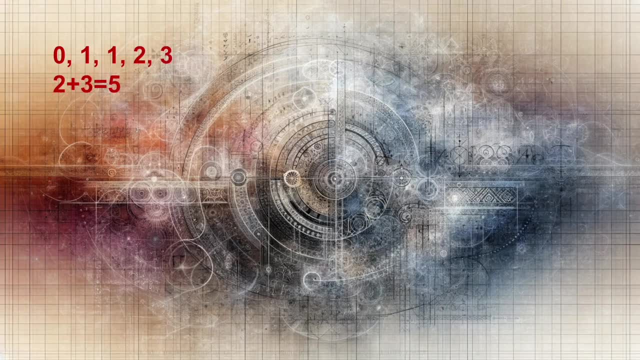 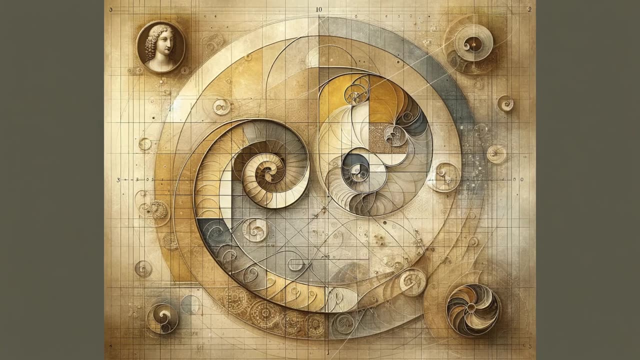 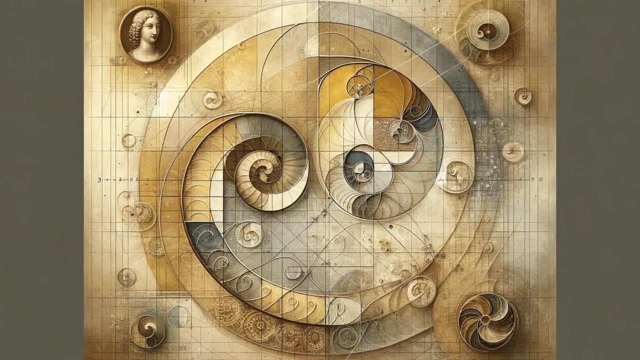 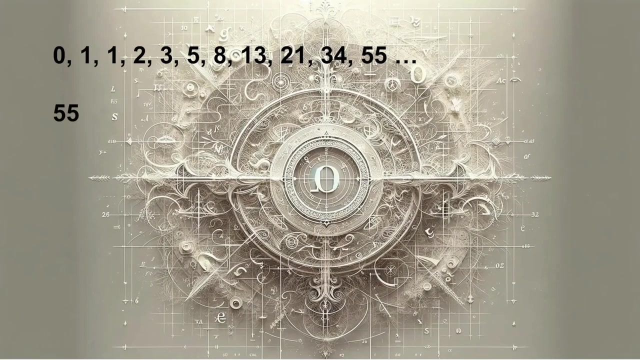 This number sequence initially emerged to model an idealized rabbit population, but over time began to be used in many areas of mathematics and science. What makes the Fibonacci sequence unique is that after a certain period, each number is approximately 1.618 times the previous number When the numbers in the sequence are divided by the. 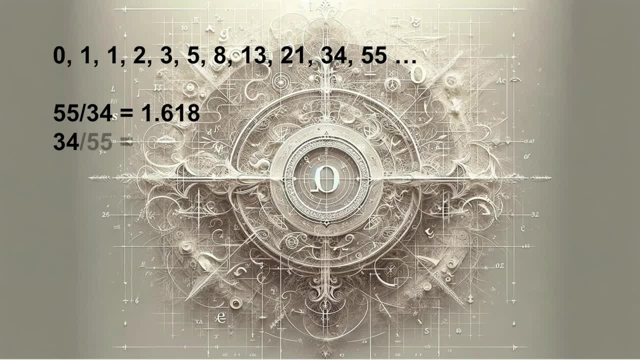 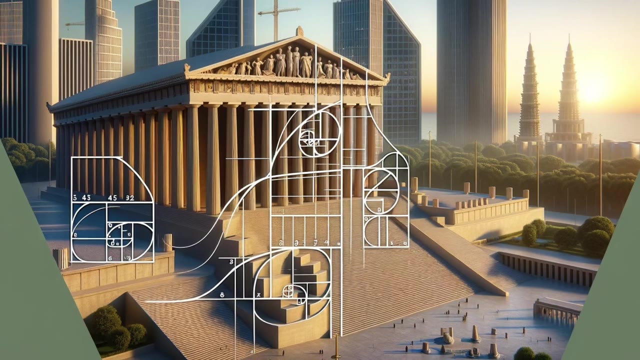 following number: the result stabilizes at 0.6 weight after a certain period. The value of 1.618 is also referred to as the phi-e number or the golden ratio. This ratio is observed in many patterns and structures found in art, architecture and nature. Let's try. 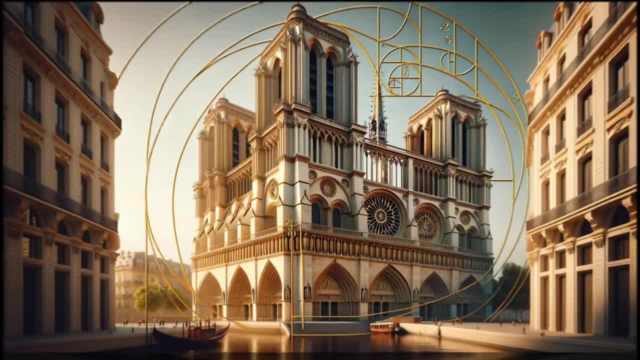 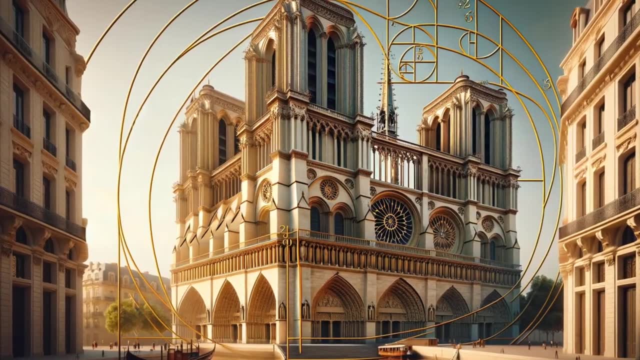 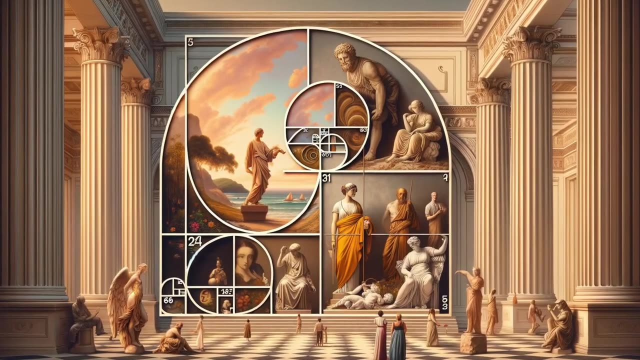 to understand how this number can be useful in financial analysis. In the financial markets, wide lengths of squares, equal to the numbers in the Fibonacci sequence, are made by placing semicircular arcs inside these geometric shapes in the opposite direction of the clock. This sequence, formed by the golden ratio, appears in many ways around the world. It is: 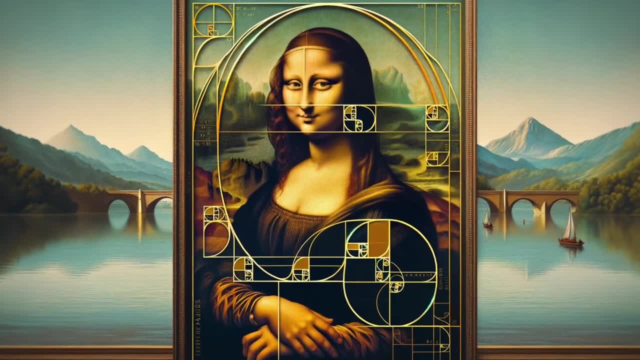 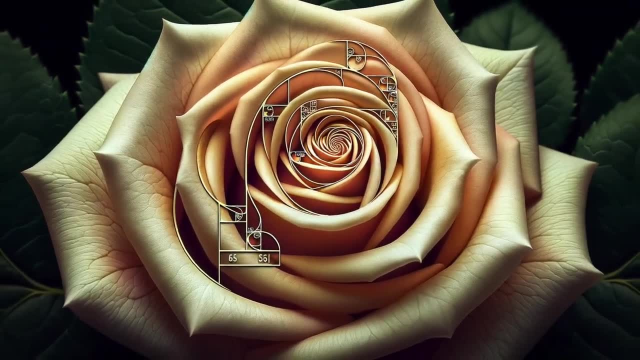 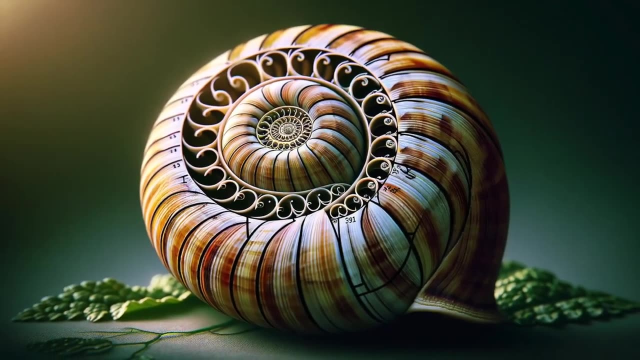 frequently observed in architecture and fine arts. For example, it has been observed in Leonardo da Vinci's painting of the Mona Lisa, in sunflowers, rose petals, snail shells, tree branches, human faces and even in spiral galaxies in space. It would not be wrong to seek a mathematical